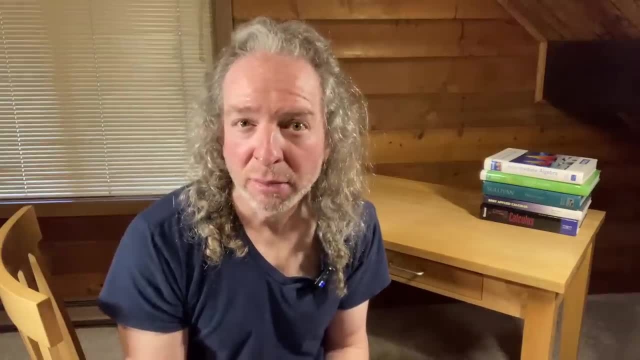 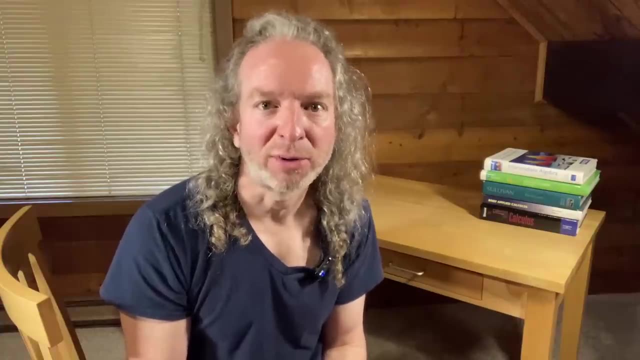 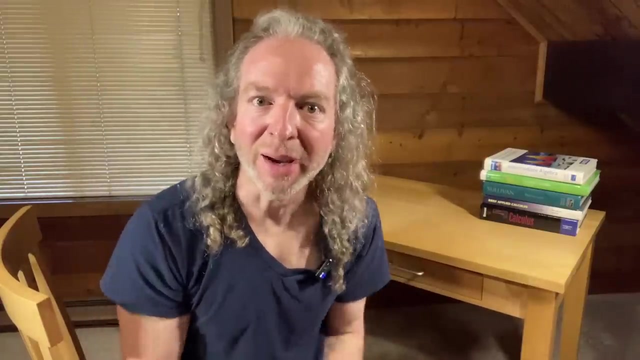 I'm waking up at three in the morning to work on a math problem that I've been working on for a week. It turns out there was a typo in the problem. I spent probably 50 hours working on one problem. What a waste of time. Now, I'm not saying you shouldn't spend some time trying to focus and 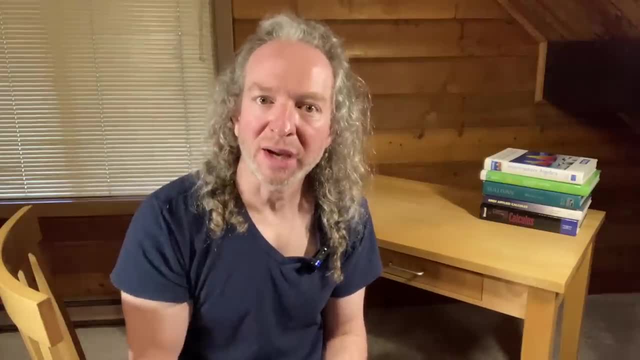 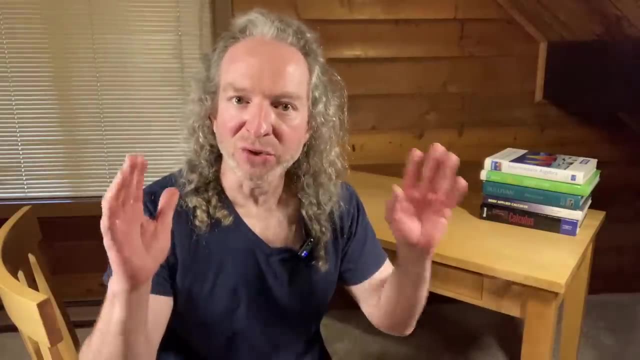 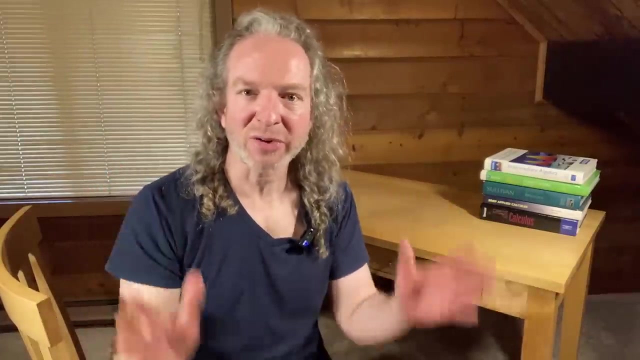 learn and understand math, But sometimes you have to move on. You have to stop trying to understand and move on and do something else. One of the things that plagues a lot of students- and I say this because I've had thousands of students over the years- is that they sometimes 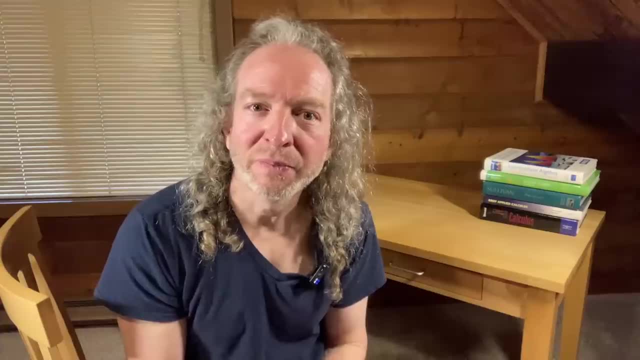 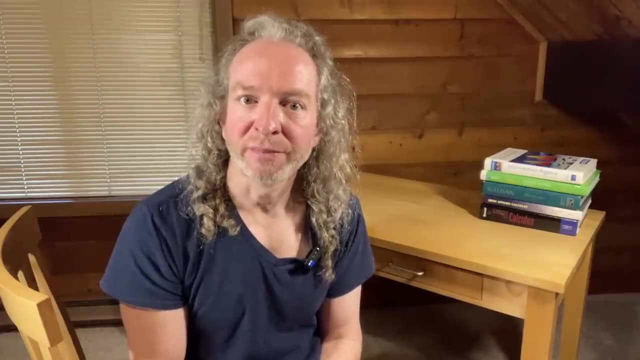 will get hung up on things. They'll get hung up on the why. They'll learn a formula in class and they'll want to understand where it comes from the derivation. They'll ask the teacher. Maybe the teacher gives them a response they don't want. They'll look in. 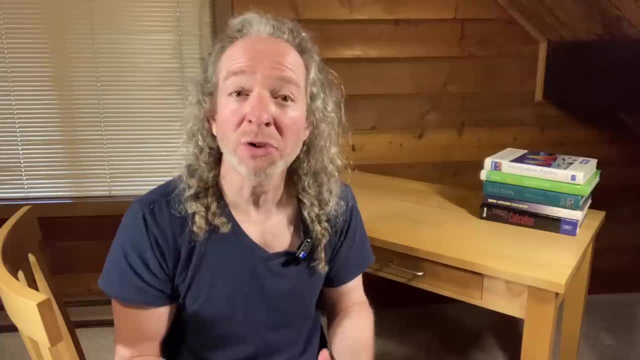 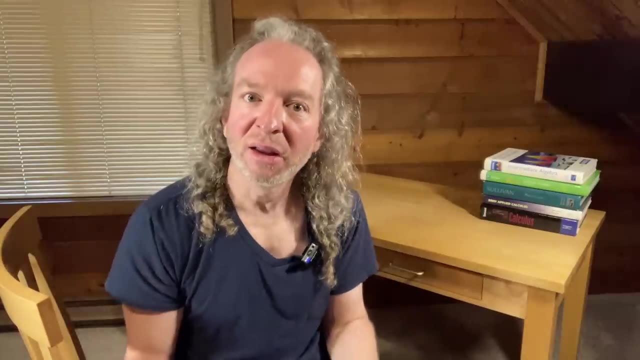 the book. Maybe the book doesn't explain it well. Sometimes they'll go home and they'll watch a video. It won't really make too much sense. They'll kind of half understand it. Hey, that's okay. Half understanding is better than not understanding at all. right, And you tried. 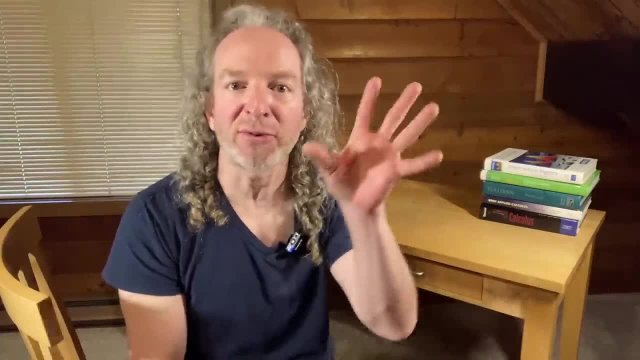 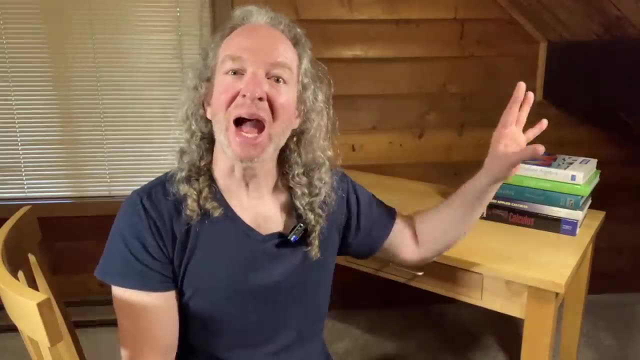 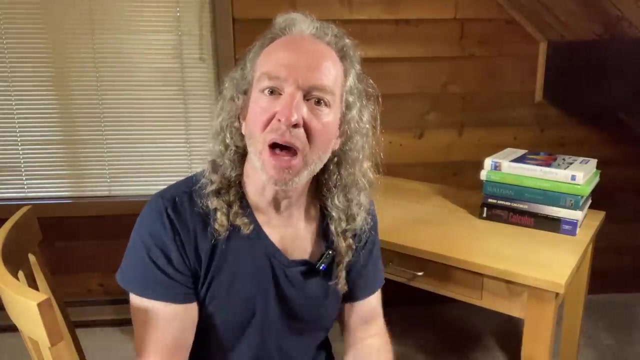 Move on right. Focus on your grades, Focus on what's in front of you right. Do what you can now Instead of spending hours and hours and hours on something that you might not be able to figure out For a very long time. a lot of times in mathematics, when you revisit things that 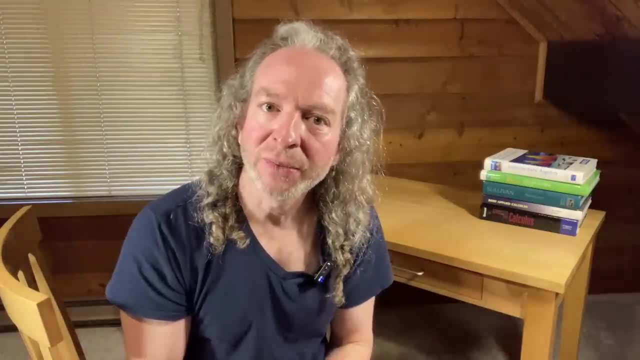 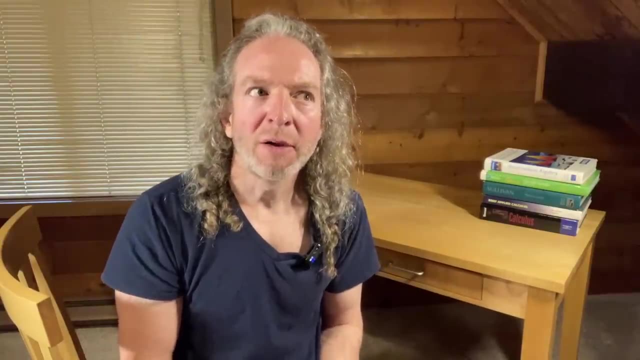 you've seen in the past, it's easier And sometimes you just don't get it. When I was in pre-calculus, I was learning about finding the inverse of a matrix. So you take a matrix and you put it into another matrix and you 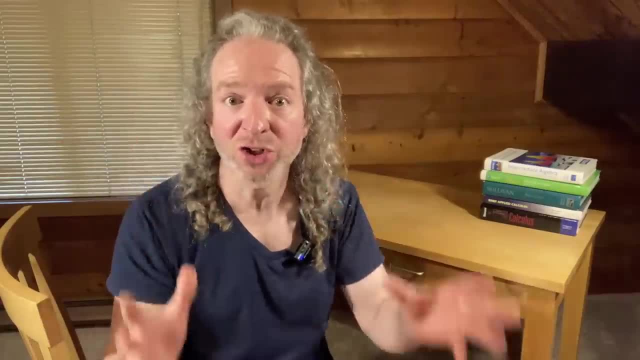 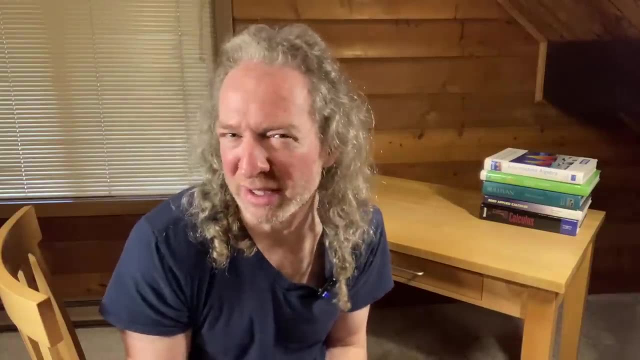 turn it into what's called reduced row echelon form. It requires a lot of practice. It requires a lot of practice. It requires a lot of practice. It requires a lot of mental calculations And I remember I had struggled with it because I always made silly mistakes And then the night before the test I stayed up till, like. 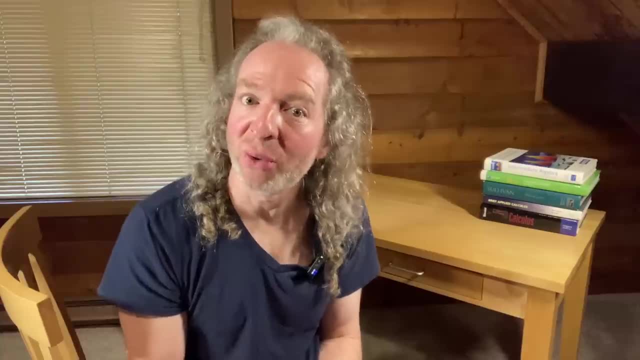 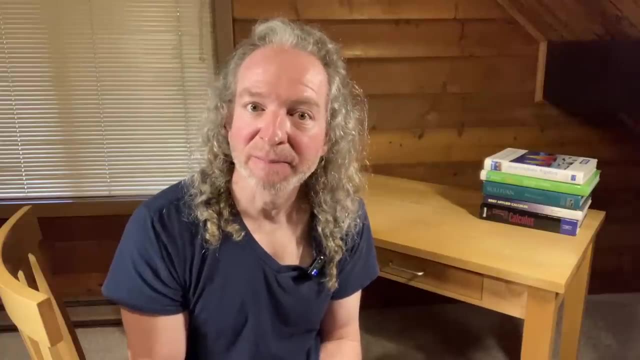 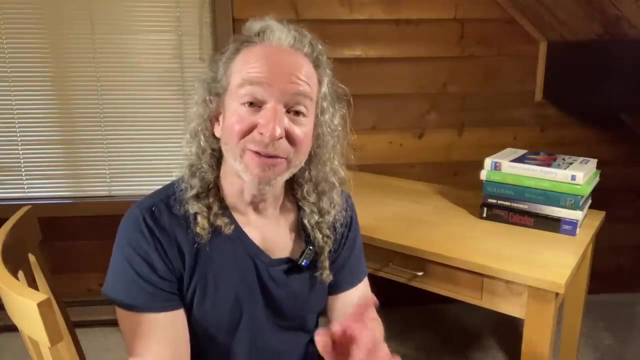 1am I thought, no, I gotta get this. And you know what I didn't? I kept making silly mistakes. Sometimes that's just how it is. Another example was learning mathematical induction with inequalities. This is a tough one And it's funny because I know it's not hard for just me. 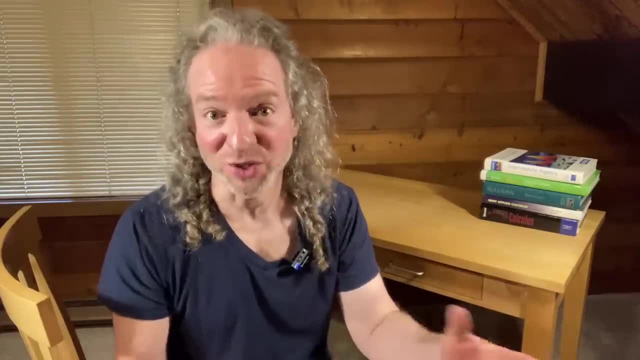 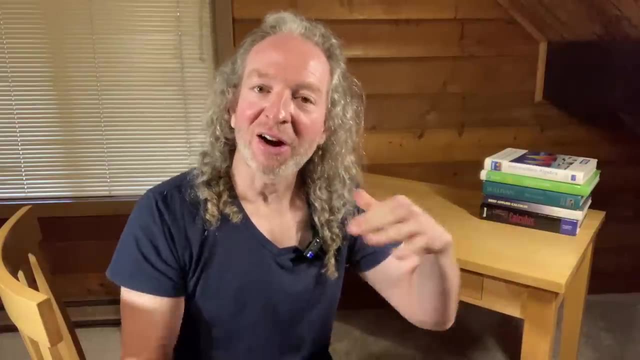 It's hard for other people And I know this for a couple reasons: 1, I've taught it in college. 2, if I look at my induction videos, I have more dislikes on the videos with inequalities. Why? Because they're harder to understand, so people get confused and they dislike the video. 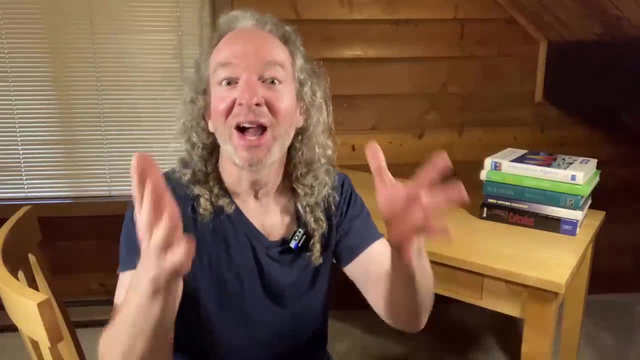 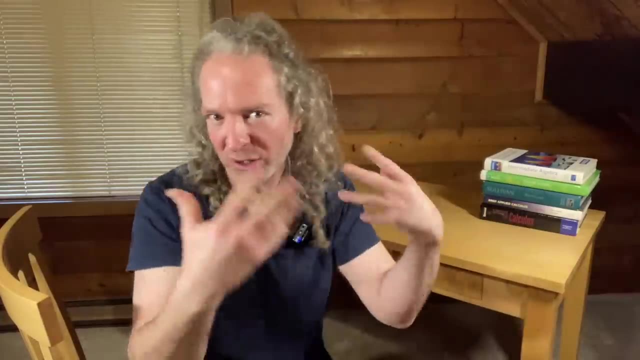 So maybe it's a bad video too. I don't think it is. I don't think they are, But I think it's because those people are having the same problem I was having, right. I mean, even though I tried to explain, they still don't understand. 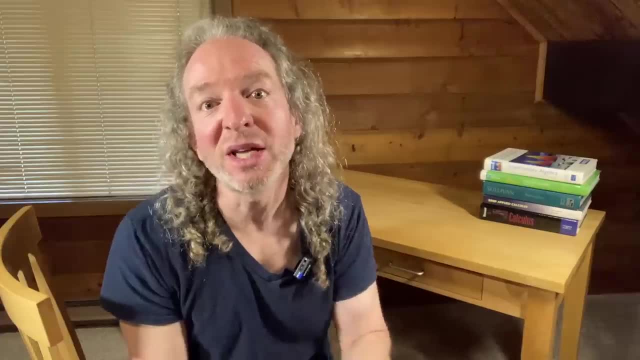 So is it my fault? is it their fault? Maybe it's no one's fault. The point is, sometimes you need to revisit things later and they'll make sense. Now. you know, those proofs are no problem for me, but I had to wait. 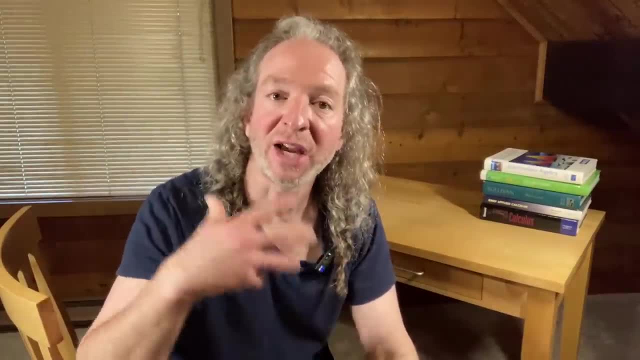 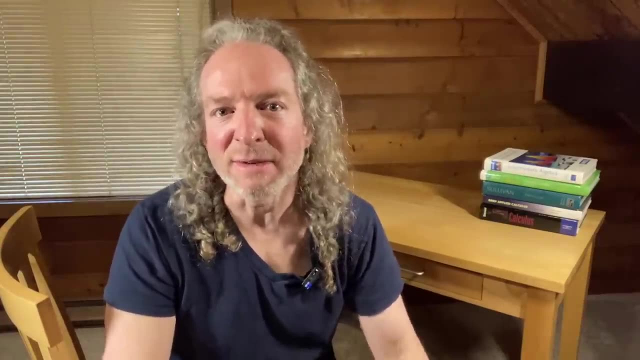 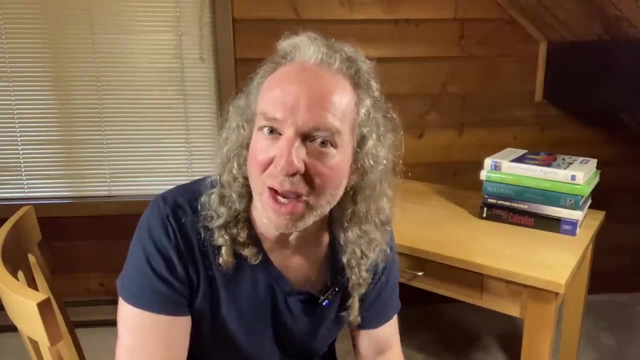 years, sometimes years, before revisiting something, and then it comes to you. it clicks. So if you're hung up on stuff, if you're hung up on some mathematics or maybe physics or whatever it is, you're trying to learn and you don't get it, it's okay, right? It's okay to not understand. 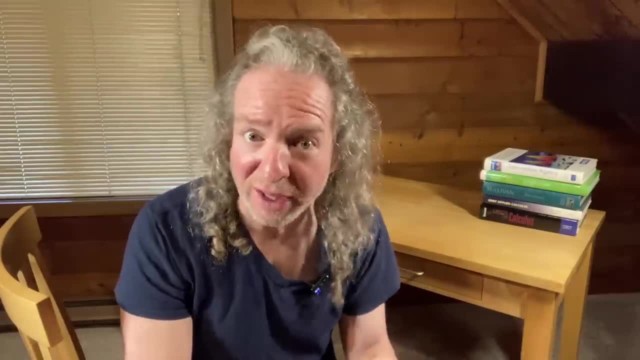 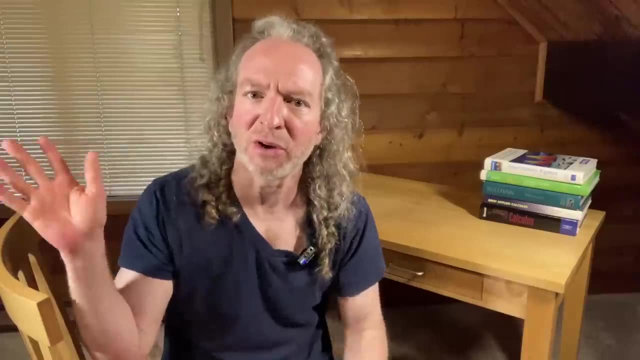 And people always put this emphasis on understanding, which is important, Like, oh you know, if you take a class, you should understand everything, And I've said this before but I'll say it again, just in case you haven't seen my other videos. But typically for me, 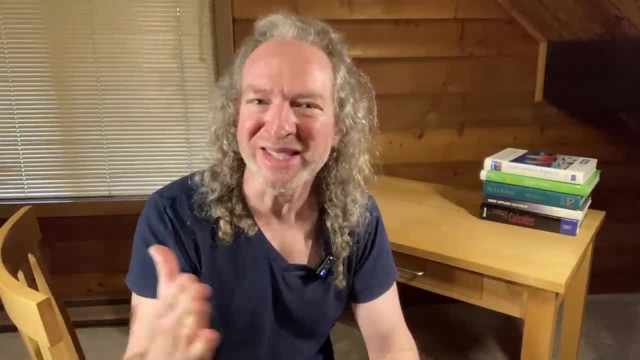 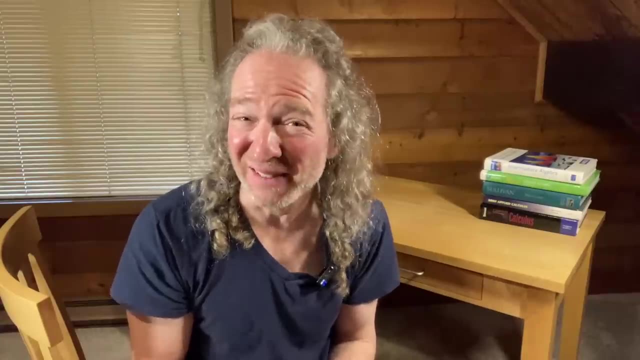 as a college student, I maybe understood 60 to 70% of what was taught in a class- 60 to 70%, And that was it. That feels kind of low to me. I mean, it feels low. I felt like I should have. 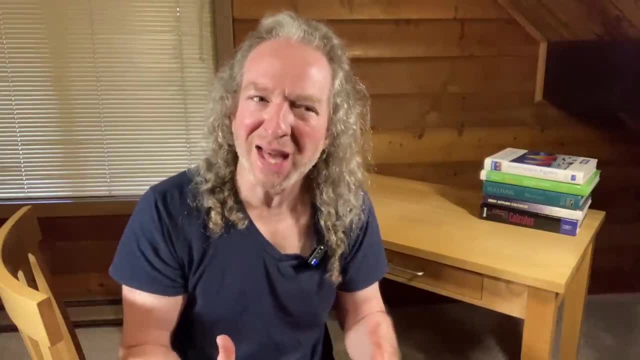 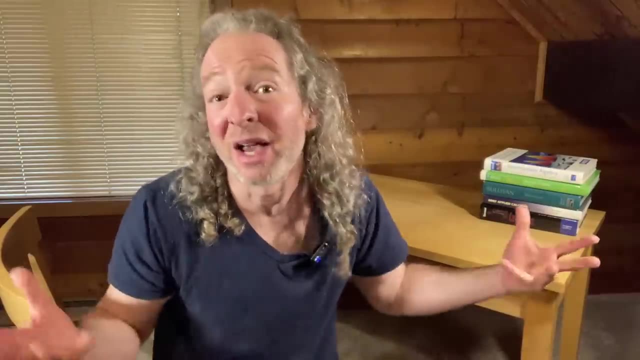 understood more. It always bothered me. I felt like I I wasn't that good. But then I knew I was good because I would go home and I would study and I would figure it out and I would do well on the test. And that's how I, I guess, would prove to. 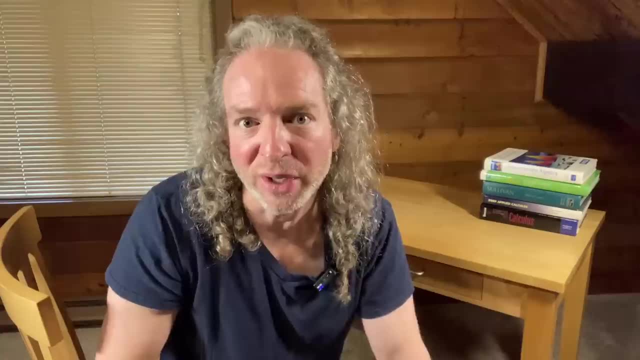 myself. if that's a thing I don't know, Not really. I just knew I could do it And so I worked hard and I did it. The point is: a lot of times you're not going to understand everything. I don't think. 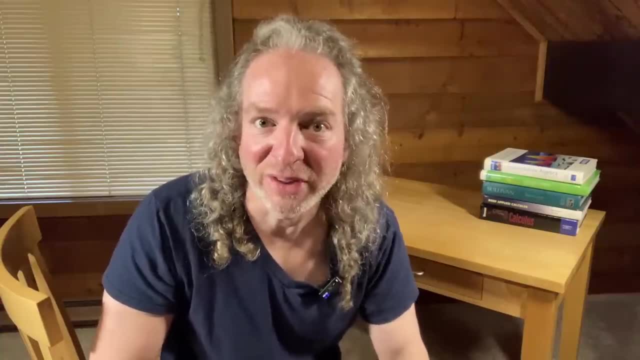 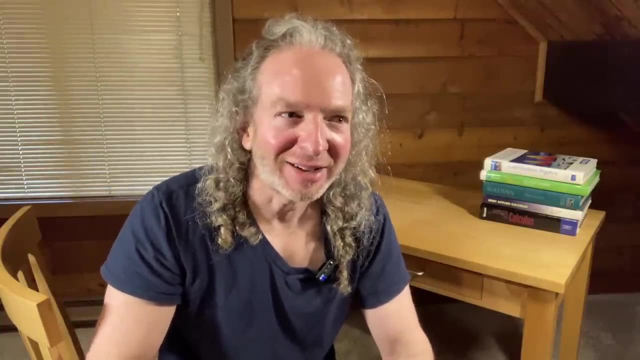 it's possible. If you take a class, I mean, it's hard to understand everything. I had a student once- Oh, he's a great guy, I just remember this story so I'll tell you really quick- And he was. 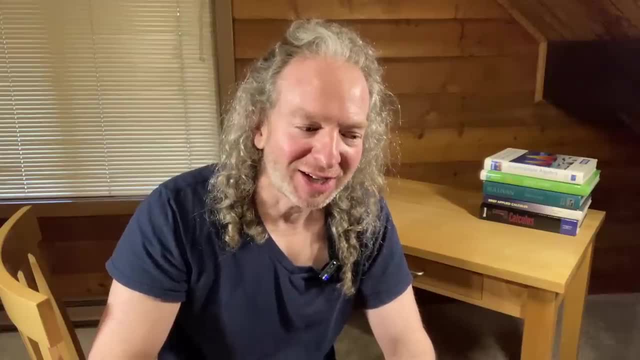 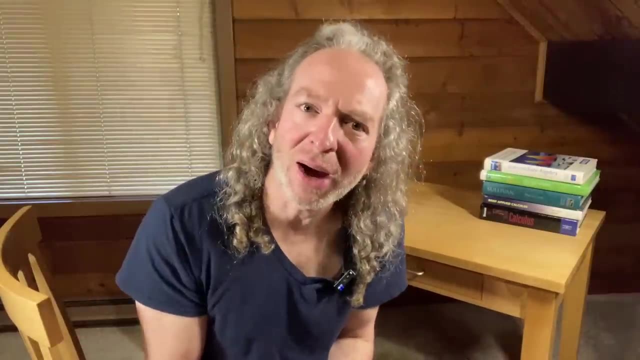 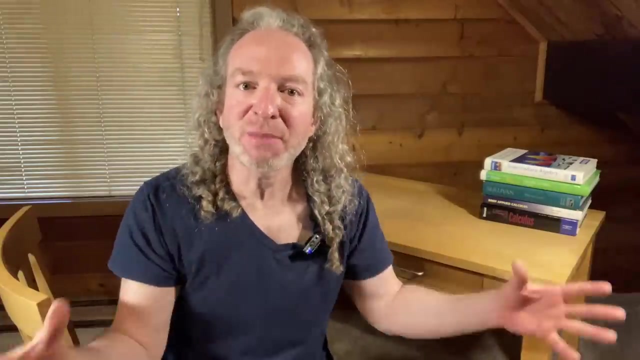 once and he said something really interesting. He said, well, a C means you understand 70% of the material, right? So that's pretty good. And I was like, wow, that's, this guy's got something right. Think about that. A C means you understand 70% of the material, So just think about any. 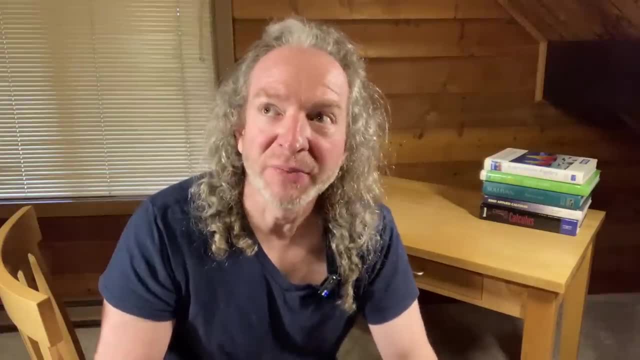 class you've gotten an A in. If I think about classes I've gotten an A in, I mean, well, I mean at the end of the class that I understand 90% or more of the material. maybe I just know. 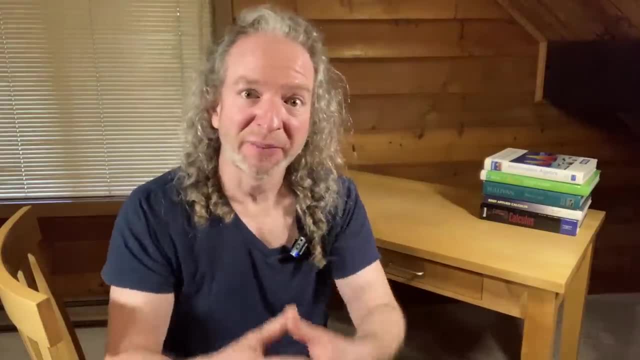 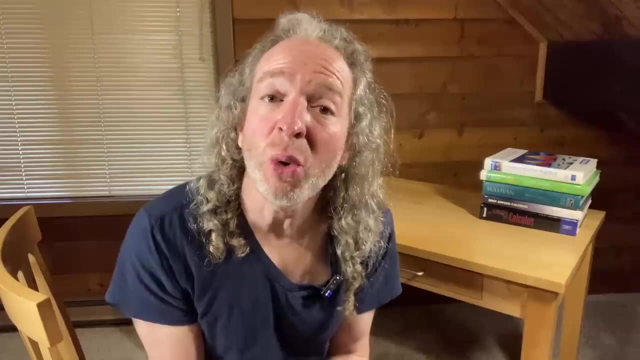 that in that lecture I caught 60 to 70% And I wonder how much people really understand when they're done with the class. Do they understand everything in the class? Probably not. So it's okay to not understand. Don't get hung up on stuff. You need to manage your time and move on. 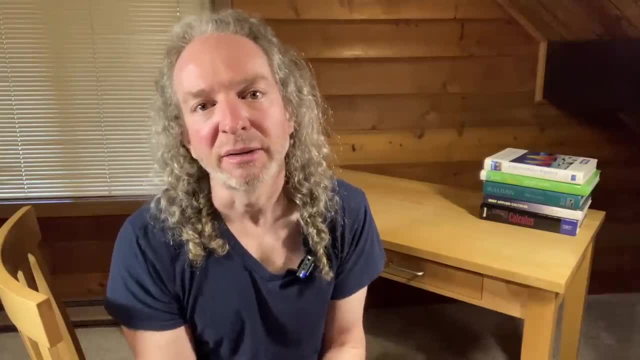 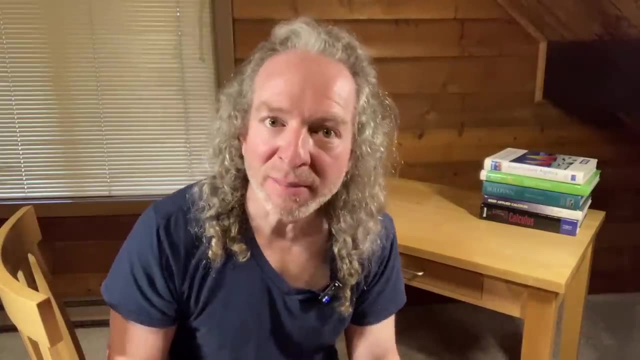 So just move on, Don't get hung up on it. Everyone struggles And if you feel like other people are getting it and you're not, it's not because you're dumb, okay, It's not because they're smarter than necessarily. It could just be because you locked the background, or it could be that. 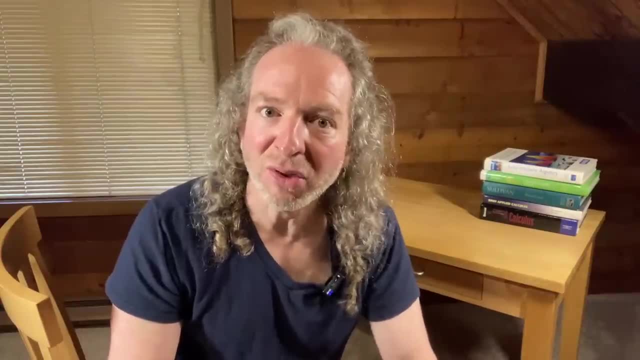 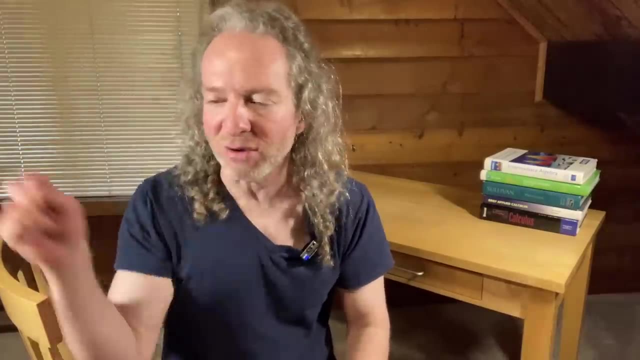 the time is just not right. You know, when I was in eighth grade I remember trying to learn algebra, copying off this kid. He would write down stuff like commutative, you know, and x plus y equals y plus x. I would just copy him. I didn't know what any of it meant. I went to the principal's. 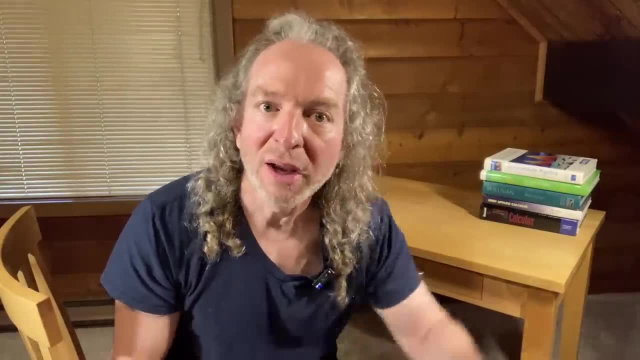 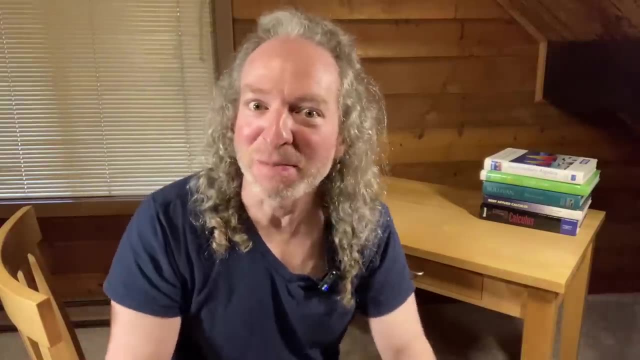 office. after class I told the principal I didn't know what was going on. They put me in a class which was horrible. It was even worse. It's like a lower level class and I didn't learn anything. So it didn't help. So that's a bad story. 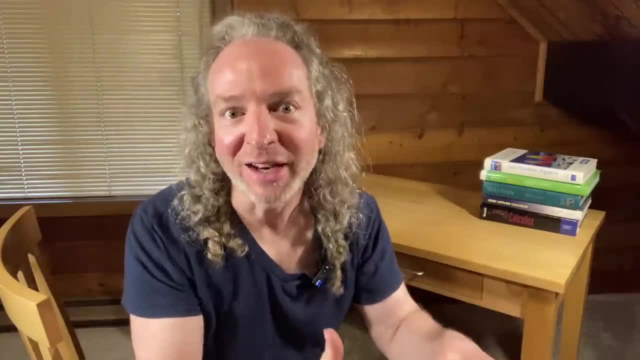 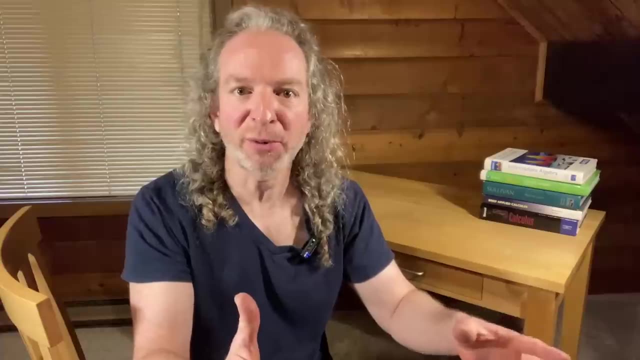 But the point was. the point is that at that time I didn't understand algebra, But later on I was able to do it. I had no good resolution then You know, going to the principal's office and telling the principal to put me in an easier class. I don't know if it helped me, I mean, 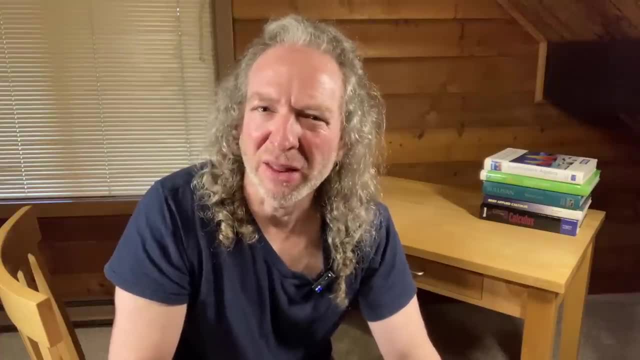 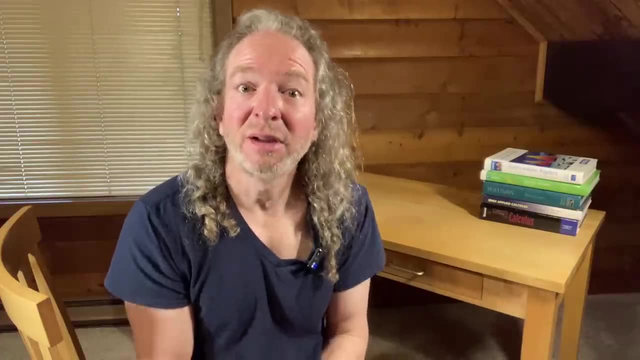 I think I passed the easier class, but I don't remember learning anything. So stop trying to understand so much and just move on when you're stuck. I'm not saying give up, but move on sometimes. And how long should you spend on a problem? you know, It just depends. 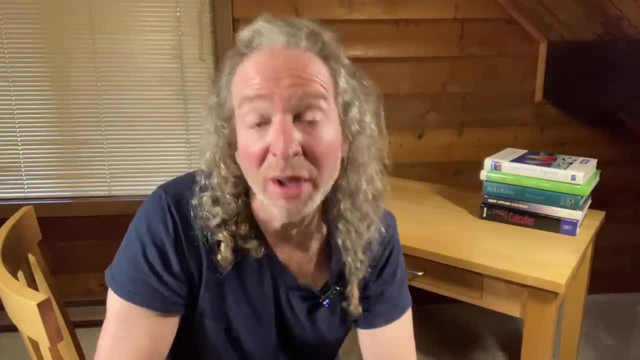 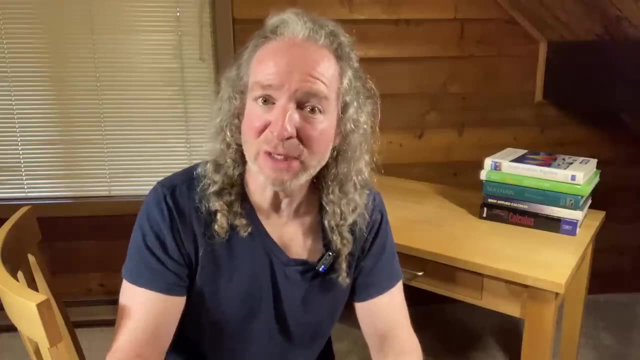 how much time you have Depends on what you're doing, right. If you're in grad school and you've got, you know, homework assignments with 10 problems, well, you know, an hour, two hours, I don't know. You can spend some time on these, right, But try to think about each problem. 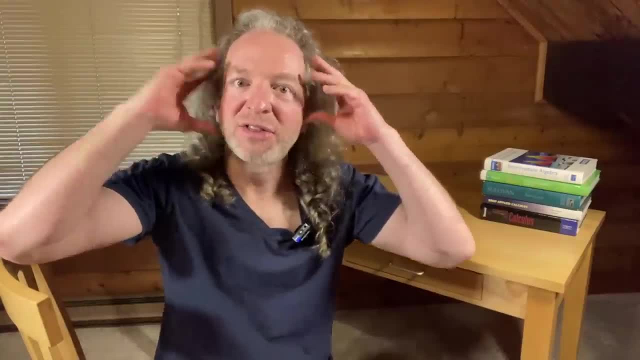 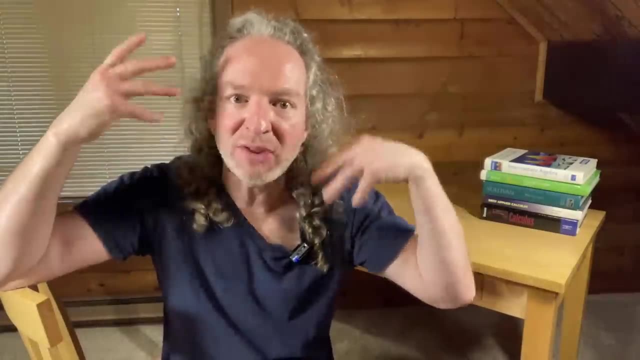 within a short period of time. So at least you have the thoughts in your mind. Read the problems, look them over right when you get them, And then the next day look them over again. You know, keep them in your mind, Keep thinking about them, you know. So look at them all. Read the questions. 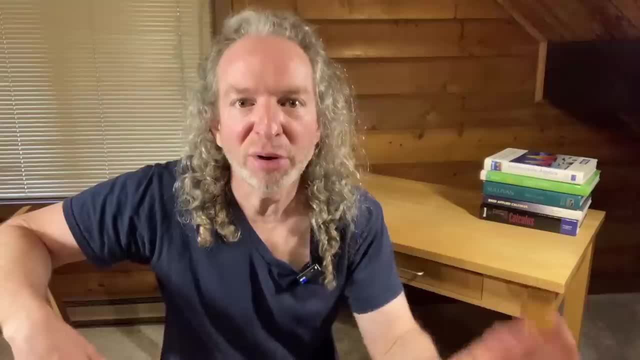 Put some effort into them And then the next day look them over again And then the next day each question, See how far you get in the proof. Put it down, then try again another day, But don't spend hours on one problem. Don't spend three hours on one problem. Don't do that, I mean. 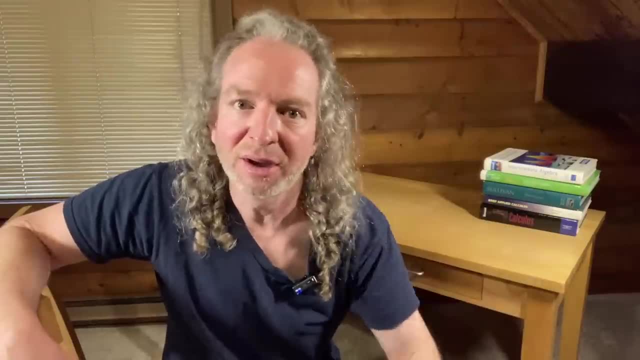 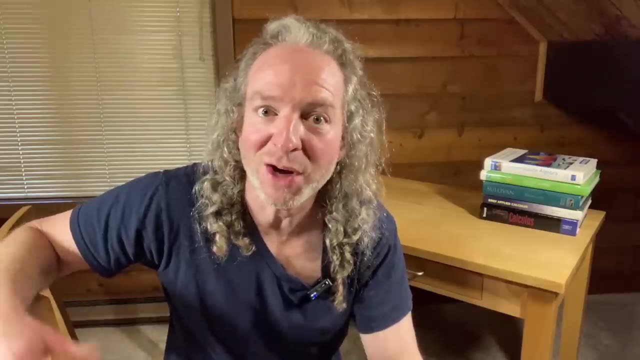 if you're doing research, it's different, But if you're taking classes and stuff, no, you can't do that right. You can't afford to do that. I should have listened to that Argentinian man, but I didn't. Hopefully, if you're watching this video, you'll take my advice. 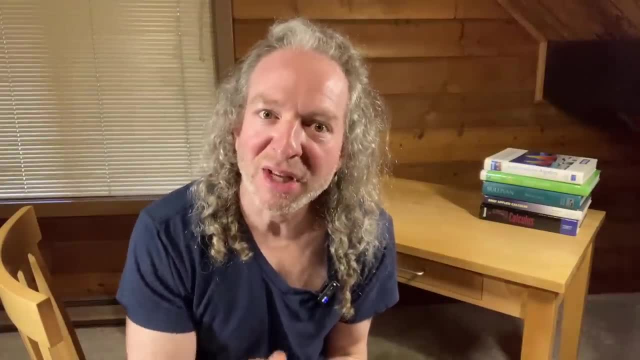 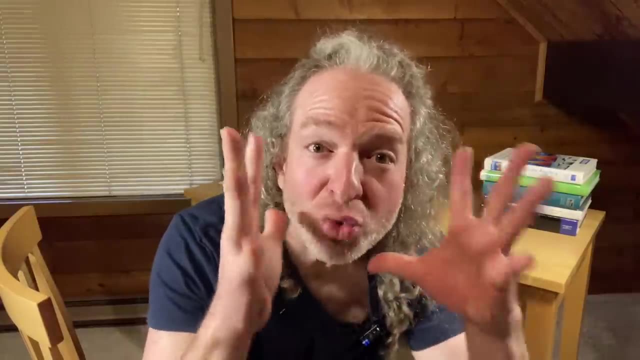 And if not, that's okay, But at least I'm trying right? Stop trying to understand so much and move on. Manage your time, especially with something so time-consuming as mathematics. It is extremely time-consuming. Anyways, if you want to learn mathematics, 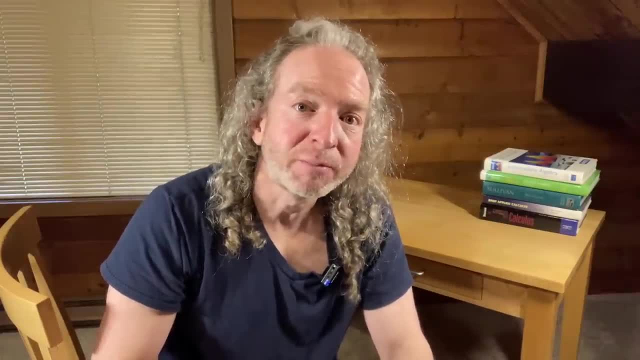 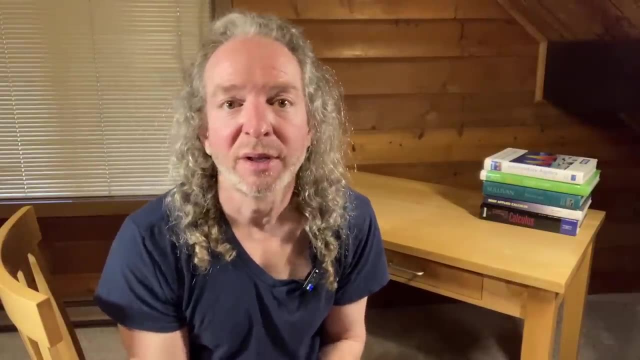 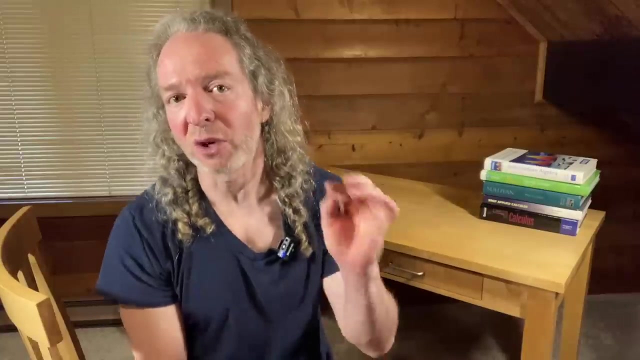 I do have courses. They're on the Udemy platform, But please use my links from my website, mathsourcercom or freemathvidscom, because, one, it helps me greatly because otherwise Udemy takes a huge cut, And two, I've lowered the price on all my courses to the bare minimum. 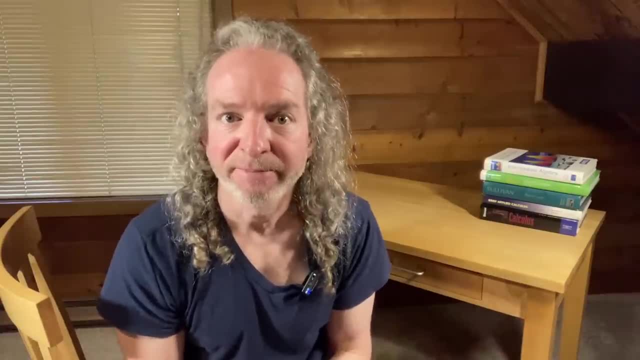 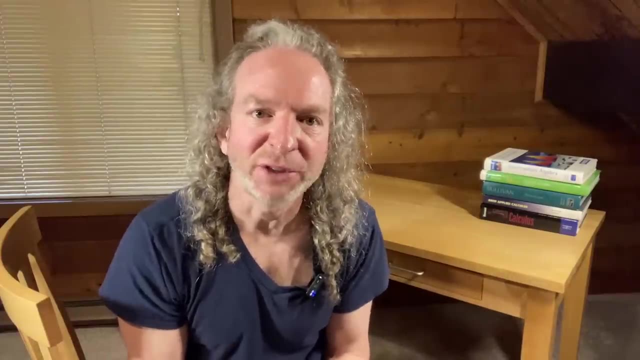 So when you click my links you should get a low price. I've got courses on algebra, calculus, abstract algebra, some advanced calculus and other stuff as well, Differential equations et cetera. I've got a bunch of courses. Some have assignments. 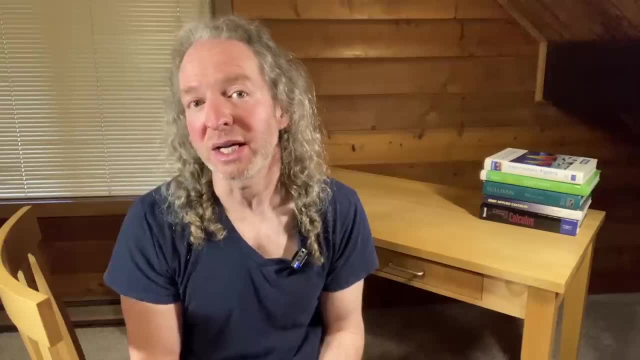 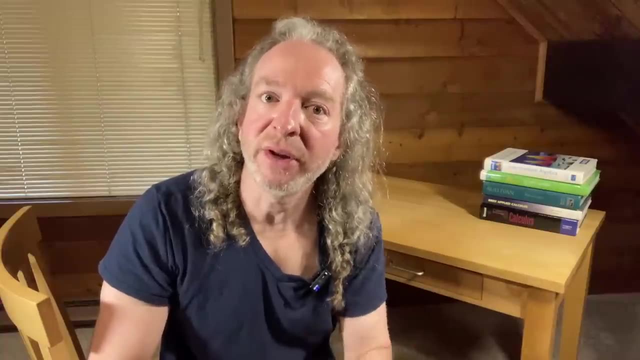 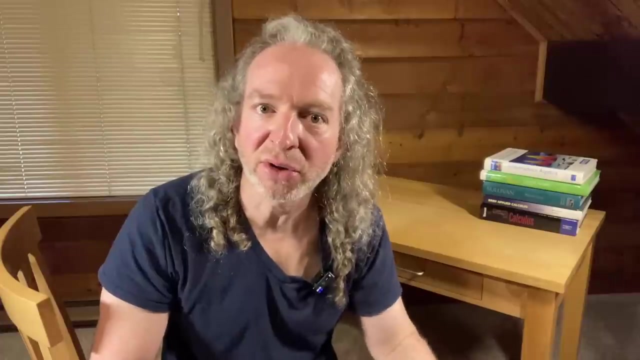 some don't. If you found any value in this content, feel free to hit subscribe if you want to. If not, it's okay too. The most important takeaway from this video, the most important thing you should take away, is that it's okay to not understand. It's part of learning.